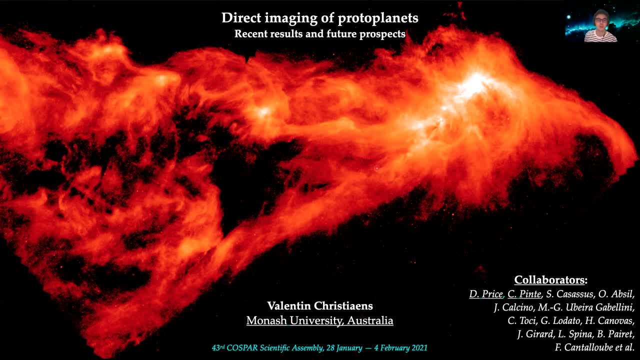 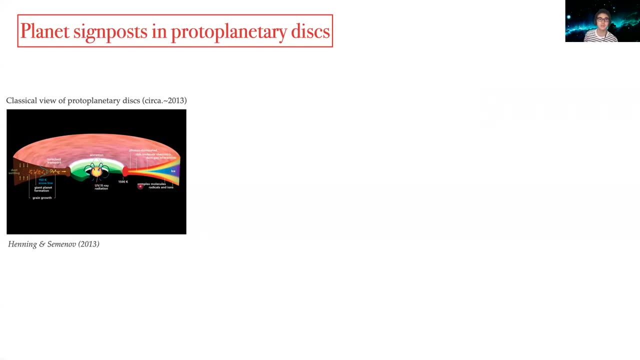 Herschel at far infrared wavelengths. So what do we know about planet formation? Well, if we zoom on one of the newborn stars in the giant clouds you see here in the background- so this is what we'd expect to see- We'd see a disk of gas and dust roughly the size of our own solar system. 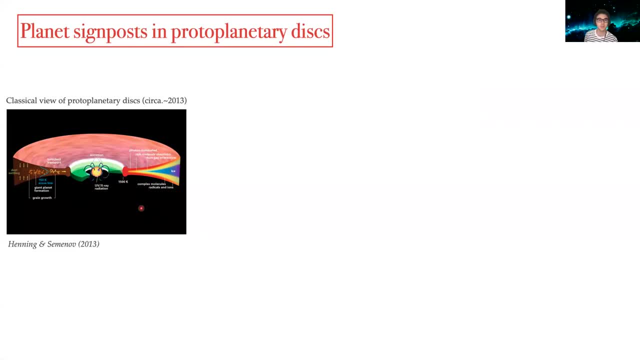 so-called protoplanetary disk in which we believe planets might be forming, And all we knew for certain until a few years back was basically that a bunch of processes must happen in the disk and somehow we end up with planets within a few million years. 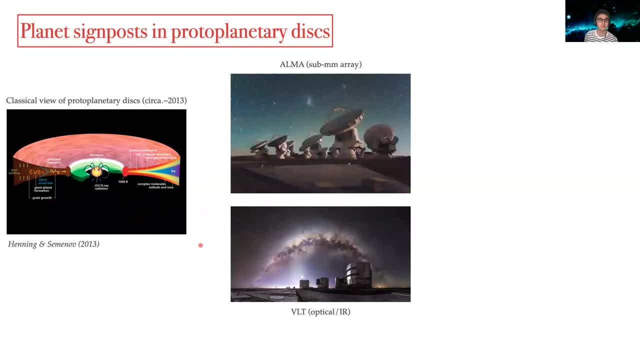 time- At least, this is what we knew until a few years ago- and in 2012, a new sub-millimeter interferometric array called ALMA has come online, and soon after new instruments like 10 meter class optical and infrared telescopes have also become available. So together this: new disk has become quite a well known and well known instrument, in my knowledge, because of our arrangement, which is we need to carry out a very precise and accurate analysis of the environment, of the environment, of the environment and of the environment, And in the energy environment, and then, as we 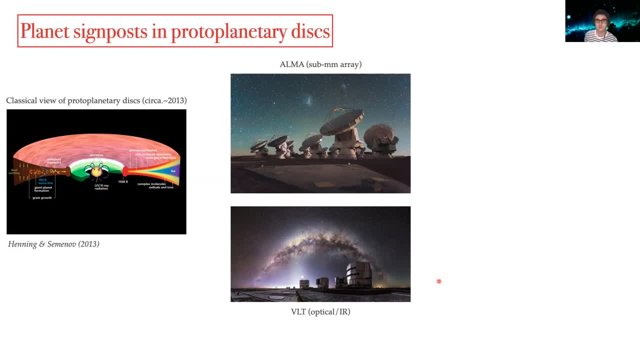 generation of instruments has revolutionized our view of the birth environment of planets. Until then, all we could see was an unresolved blob corresponding to this disk. And now we've been able not only to resolve the disk, but actually to completely change the picture and to image a number of 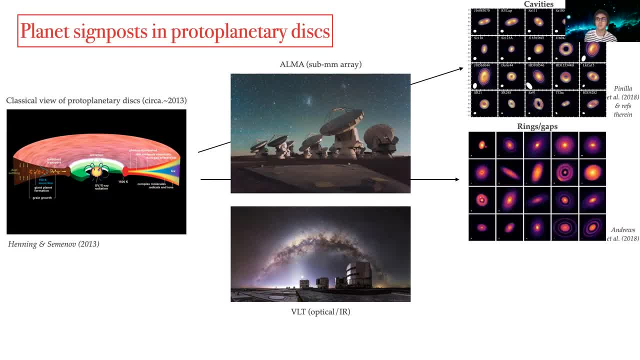 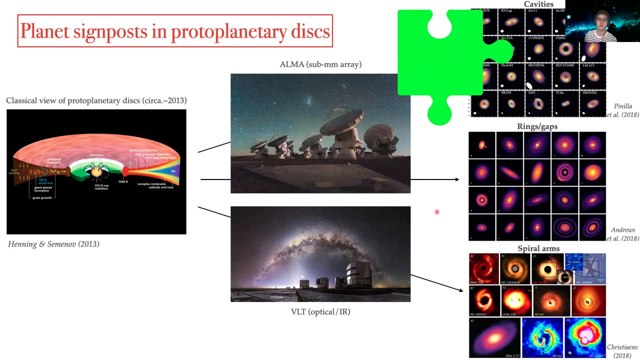 substructures in those disks, including cavities, rings and gaps or spiral arms, And all these structures may point to the presence of companions in this disk. So we've been gathering these new observational pieces to the puzzle of planet formation, But now we need to directly image. 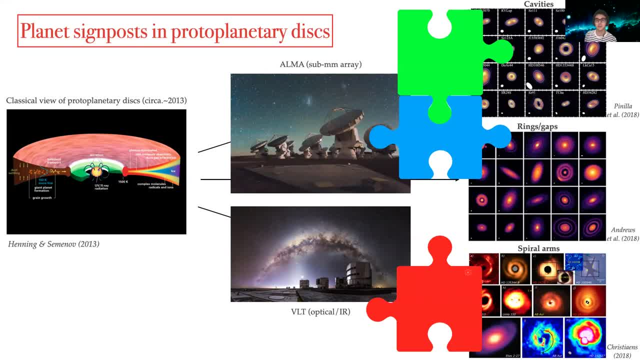 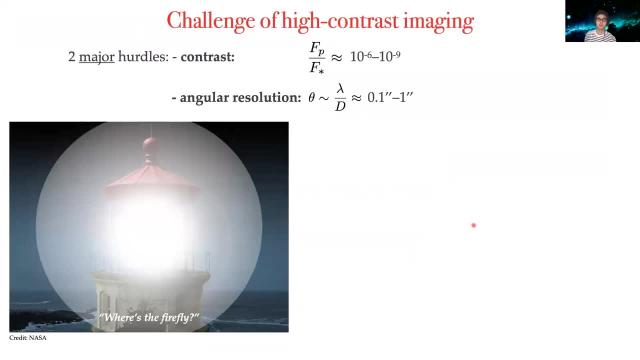 these protoplanets, to connect the dots and understand precisely how these structures are connected to embedded planets and what they tell us about the formation process. So how can we do that? Planets are much fainter than the star they orbit. They can be. 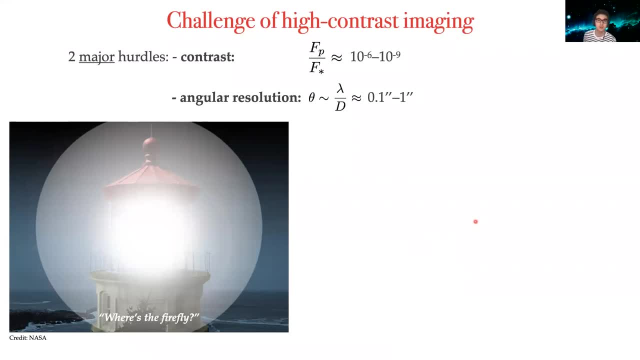 up to a million or a billion times fainter than the star, depending on the wavelength and the age of the system, And in addition star forming regions are relatively far away. So to probe astronomical unit scales one needs an angular resolution better than a fraction of an arc second. So this is a very 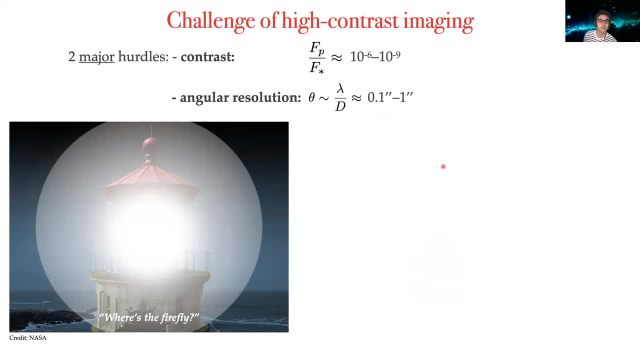 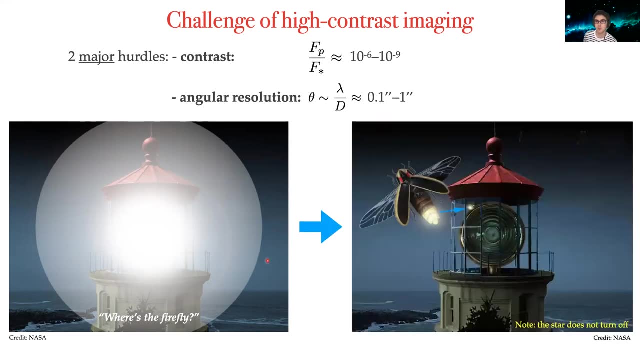 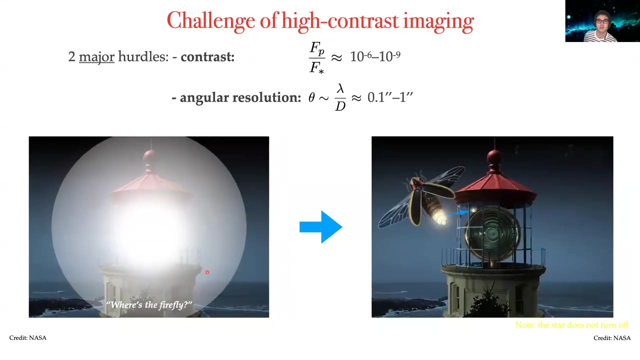 challenging task to to image. It has been compared to trying to image a firefly one meter away from a lighthouse. Unfortunately, we haven't found the switch for stars yet And since stars are far away from us, this is for trying to image a firefly one meter away from a lighthouse. 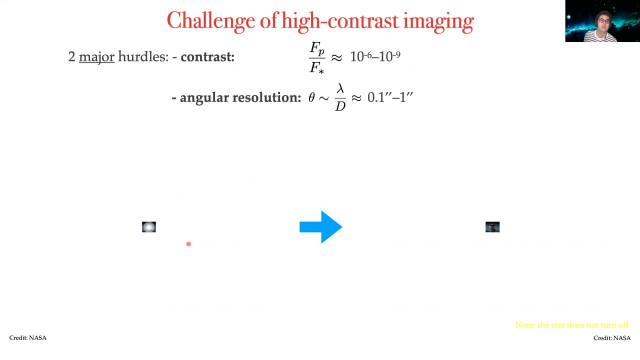 that is located 1000 kilometers away from us. So fortunately newborn star- sorry, newborn planets are expected to be brighter in the infrared and a bit easier to detect. So one still needs to reach a high contrast, the other of 1000 or 10,000.. So how does one reach such? 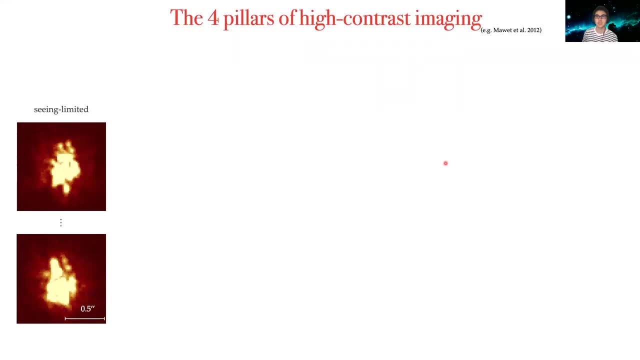 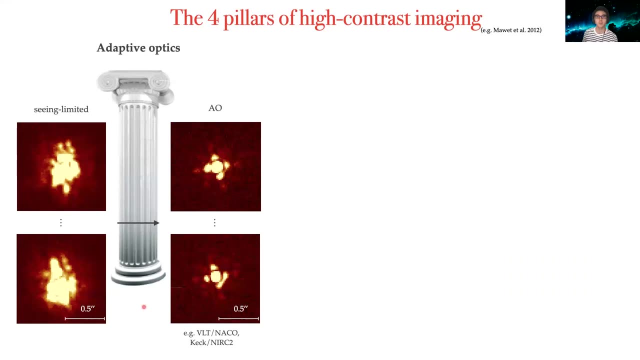 high contrast at high angular resolution. Well, there are basically four pillars to high contrast imaging. The first pillar is adaptive optics, which corrects for atmospheric turbulence in real time. So you have a more point like point spread function for the star. So this: 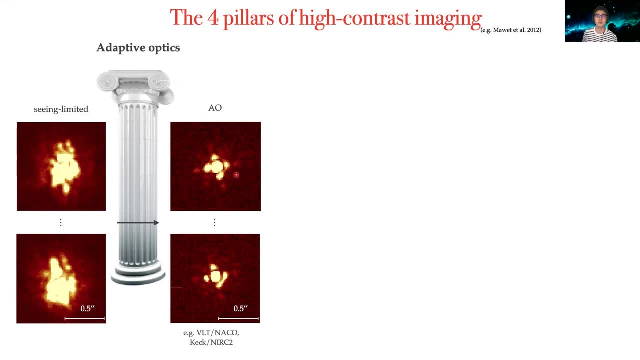 helps you reach a high contrast at high angular resolution. And this is the kind of image you get for first generation adaptive optic instrument. But nowadays we get with the latest, latest generation of adaptive optics instruments or extreme AO instruments, this kind of images where we get much better stability of the point. 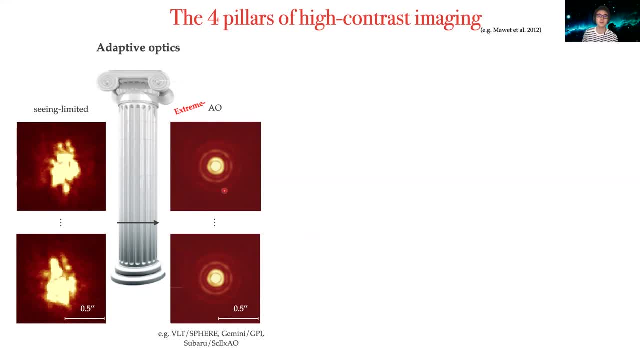 spread function. So this is the kind of image you get for first generation adaptive optics instruments. But nowadays we get much better stability of the point spread function And we can even see several airy rings in the PSF. So that's, that's one, One first step. So the second pillar is: 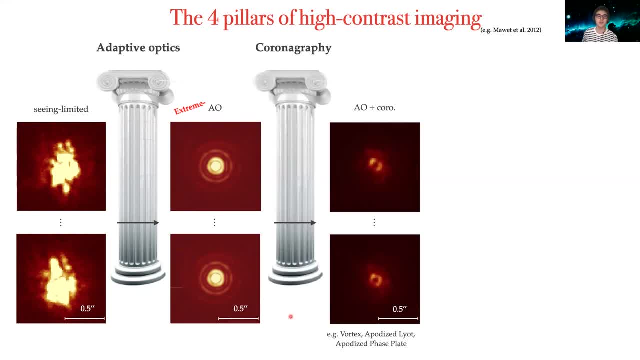 coronagraphy. So a coronagraph is a device composed of several optical elements, such as a physical mask and a Leo stop that are placed in the optical path coming out from your telescope, And a lot of design of coronagraphs, But the point they share in common is the 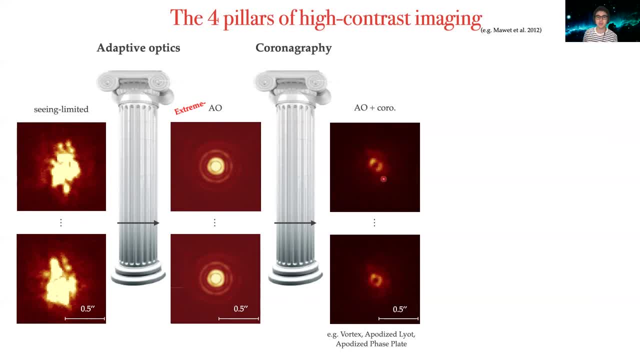 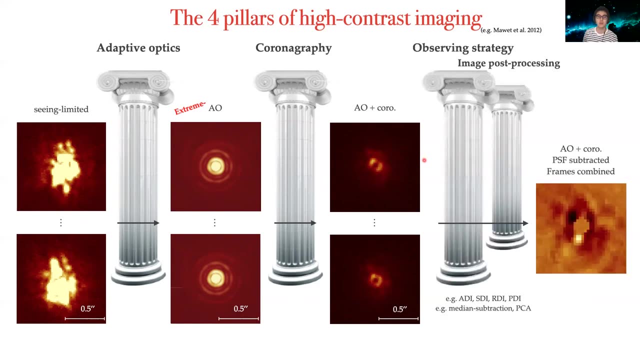 constellation of as much of the light from the star while preserving as much physical signal from its vicinity. So so, basically, this helps to reach a higher contrast in the vicinity of the star. The third and fourth pillars are entwined and consists in a relevant combination of observing. 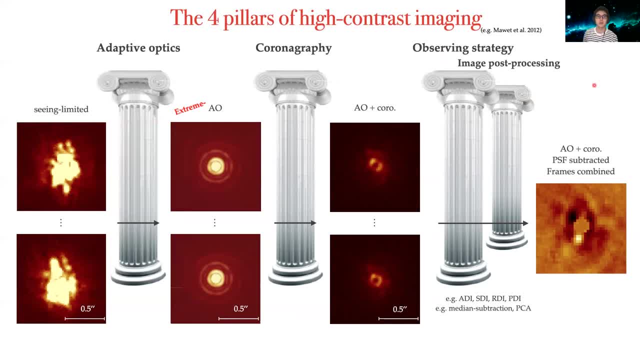 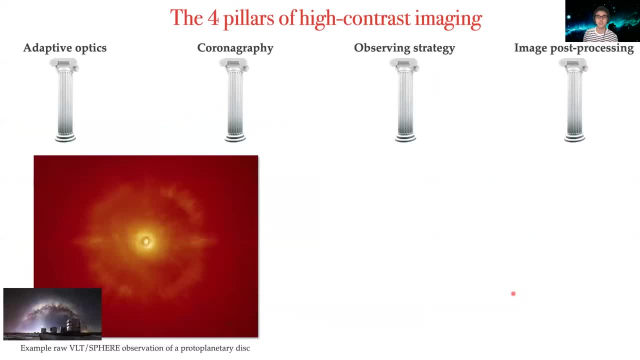 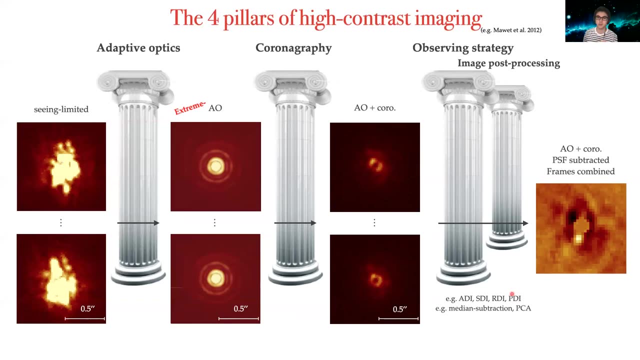 strategy and image post processing algorithm. So observing strategies include angular differential imaging, spectral differential imaging or parametric differential imaging. So I won't go into the details of those strategies, but they all share in common the goal of isolating sick and stellar signal. authentic signal, bit disk or 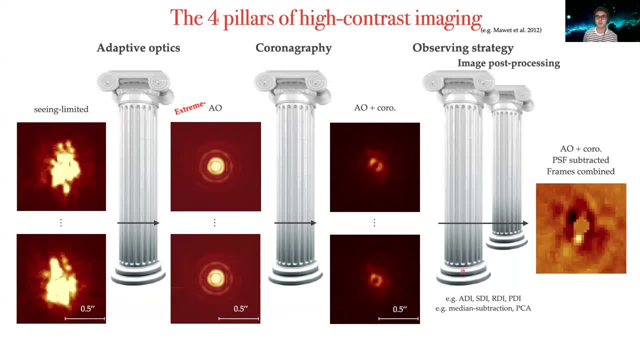 planet, signal from spurious spec, speckle, signal from the star in one way or another, And the post pressing algorithm leverages on this diversity to model And subtract the emission from the star without subtracting the emission from a planet or a disk. So the aggregate finally combines. 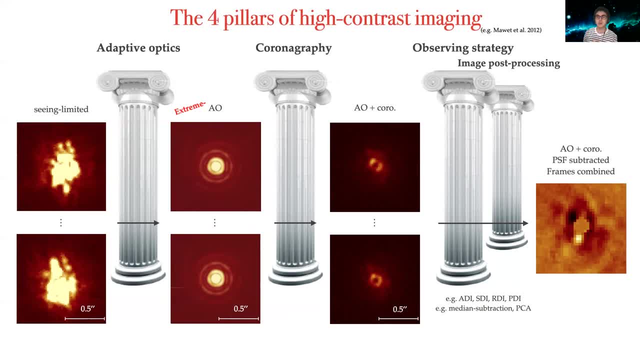 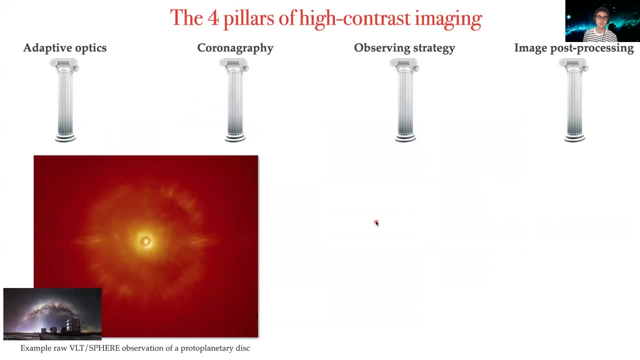 all the residual images where the star has been subtracted into a final image attached, such as this one where you're left to assess whether your residual signals are authentic or tracing artifacts. So, using these four pillars, one can effectively turn off the lighthouse. 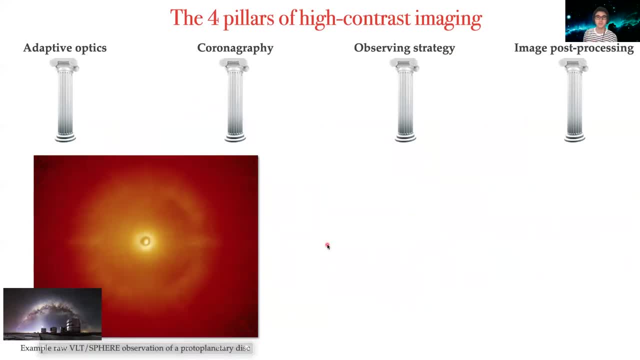 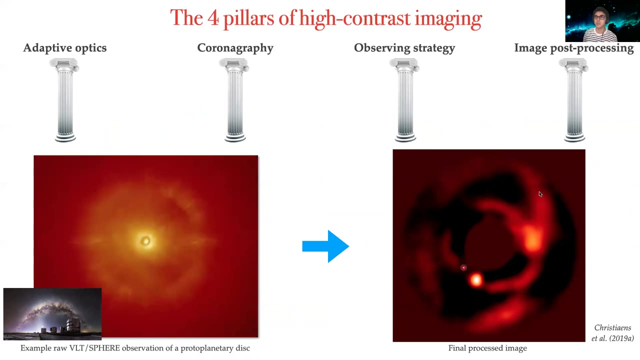 and go from this row. adaptive optics fed sighting emails circa. stop using Karena graphics sequence of images obtained by sphere, the veneer telescope. so one can go from this to this kind of final image on the right in this case, showing the pds 70. 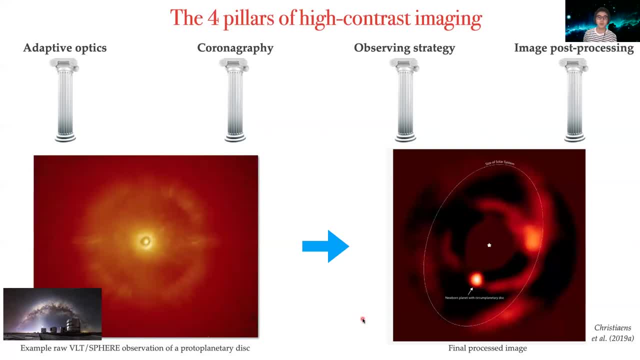 system. So this system is the first and so far only system with a confirmed direct detection of a planet. So there have been a number of other perturbanal detection claims the past decade. however, most of them either need further confirmation or have already been shown to. 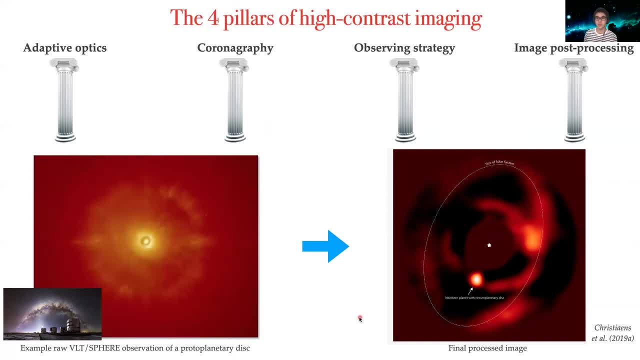 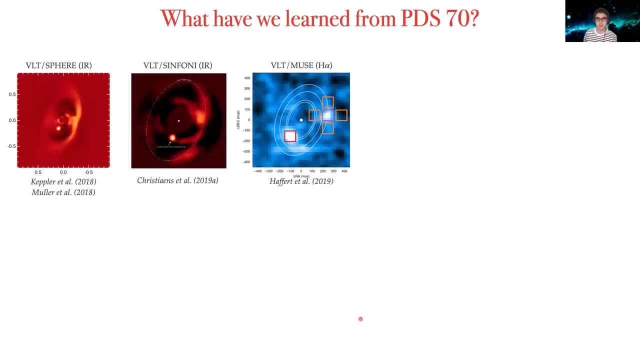 trace extended circumstantial test signals that have been filtered into a point source by the post-processing algorithm. So let's dive a bit more onto PDS70 and see what we have learned so far. So Planet B was first detected at infrared wavelengths by two independent teams. 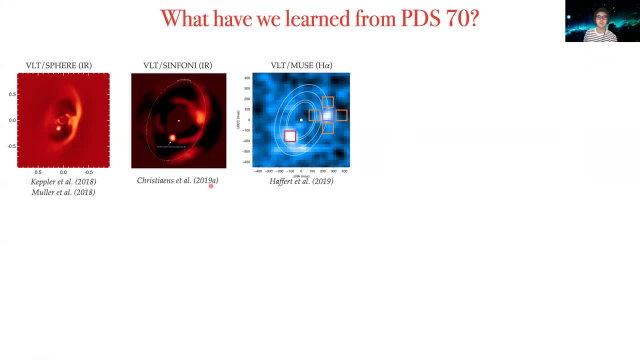 using two different instruments, and it was then confirmed to emit a significant H-alpha signal. So the H-alpha line is a known tracer for hot gas being accreted onto either planet mass or stellar mass companion, And we can see in this image that there are two. 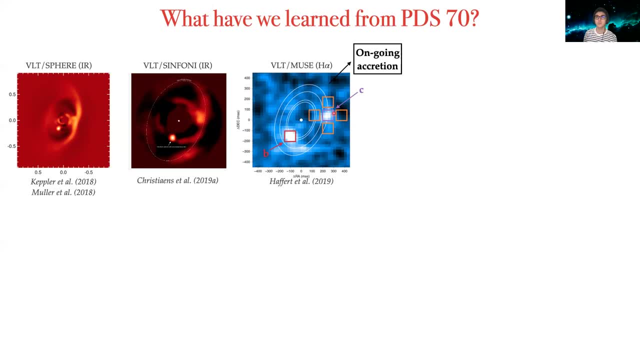 point sources, not only one for B, but another point source that suggests a second protoplanet is present and accreting material. So by measuring the flux of Planet B at different wavelengths in the infrared, we've assembled a spectrum which we have compared to atmospheric models and circumplanetary disk models. and 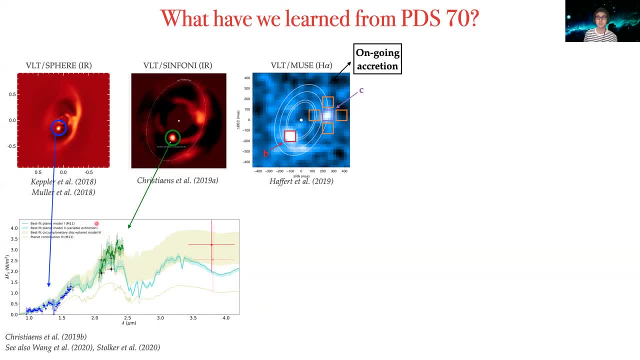 we found it was that the observed spectrum was best reproduced using circumplanetary disk models. So this was the first evidence, observational evidence for the presence of a second planetary disk. and those circumplanetary disks had been predicted for a long time as being the expected. 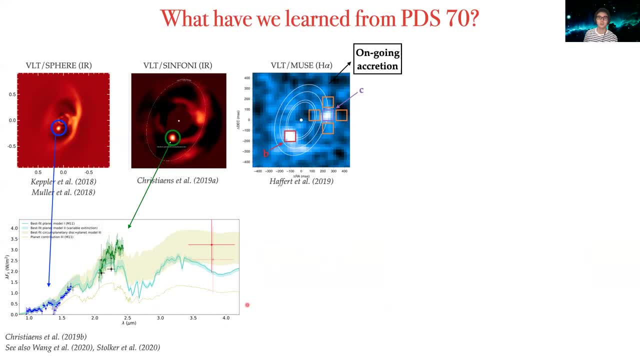 location for the formation of regular moons around the planet And, as a matter of fact, the latest observations at 3mm wavelengths were, with ALMA, confirmed emission from both location of B and C And, since the millimeter observations are sensitive to thermal emission from large. 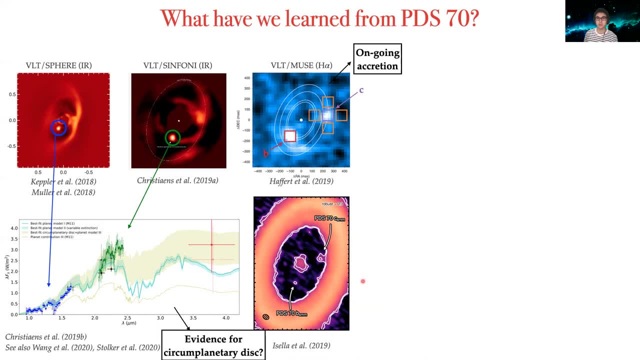 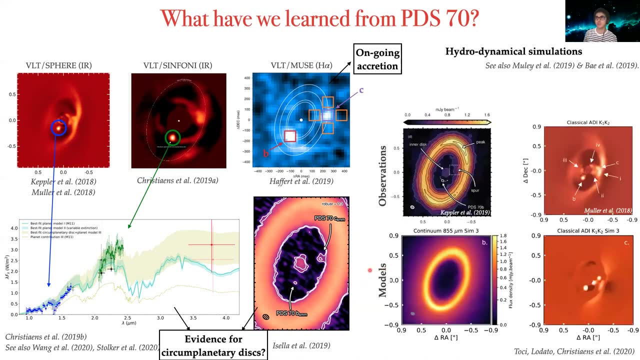 dust grains. this provided additional evidence for a second planetary disk around each of the two planets. So we have recently performed 3D hydrodynamical simulations of this source using PHANTOM, a code developed by Daniel Price here at Monash, and we plugged the result of the simulation. 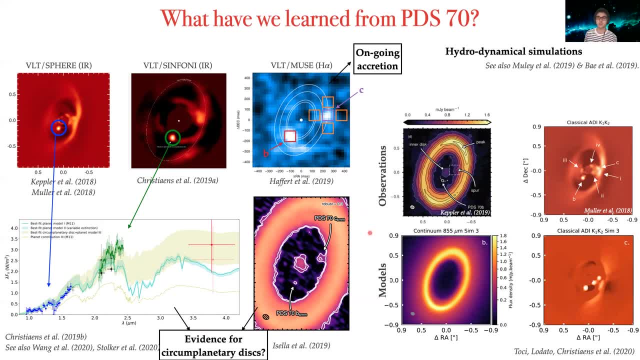 into a radiative transfer code to predict images at submillimeter and infrared wavelengths. Furthermore, for the infrared image, we post-processed the predictions using the same algorithm as the ones that were used in the observation, And this is to compare apples with. 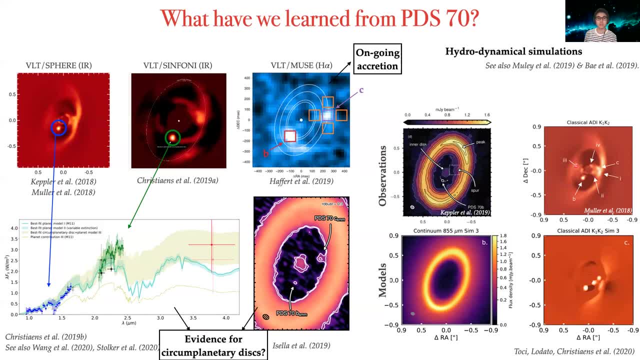 apples. since we know these images are affected by geometry biases due to the post-processing algorithm, We can see we're reproducing quantitatively most observed features, so the large cavity spur and most of the features observed in infrared. So the agreement is remarkable, considering the freedom in the initial conditions of our 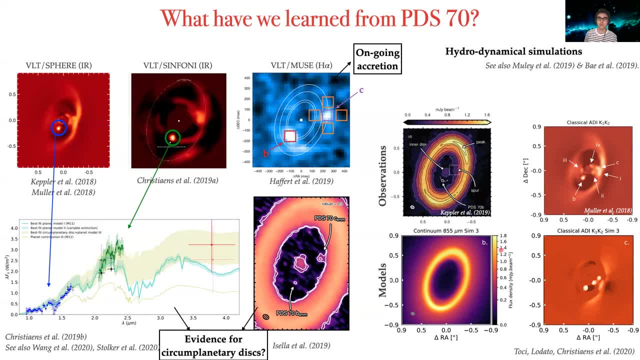 simulation. So we started the simulation by only injecting two planets at large separation in the outer disk. We let them free to migrate and then create material to grow, And we let the simulation run for a few hundreds of orbits And we see the planets migrate inwards. 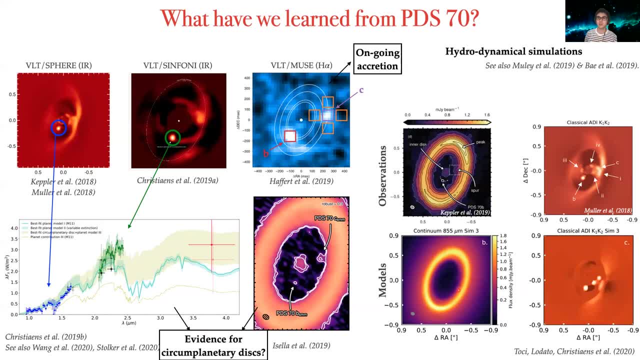 I create a few Jupiter masses of material and then they lock themselves in resonance at a similar location as what is observed. So this shows that the PS70 system appears to be a natural outcome of planet migration, followed by resonance locking. So let's now have a quick look at 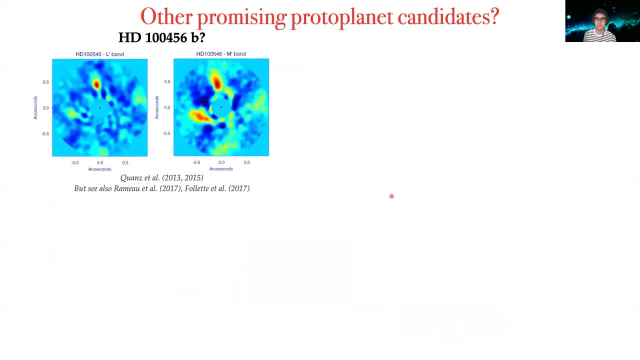 other promising protoplanet candidates that still require confirmation. So there's a protoplanet candidate in the disk of SG1456.. As you can see here, a bright signal at a terminal infrared wavelength which appears to be slightly extended to, but it is still unclear whether this is indeed tracing a protoplanet or a filtered disk signal. 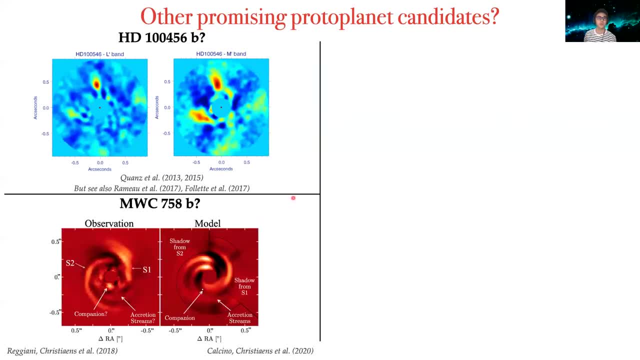 So another protoplanet candidate was found in the system of MWC758.. So we found in 2018 in those infrared observations a point-like source relatively close from the start, about 20 AU from the start. So we detected it at two different epochs And then recently we performed hydrodynamical. 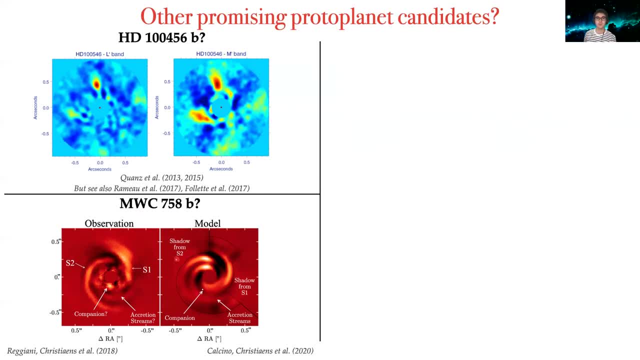 simulations to reproduce these features. So at two millimeter wavelength we also see a large cavity. So with our hydrodynamical simulations, in which we injected a five Jupiter mass planet on an eccentric orbit, we can reproduce both the observed spirals and the cavity. And, interestingly to 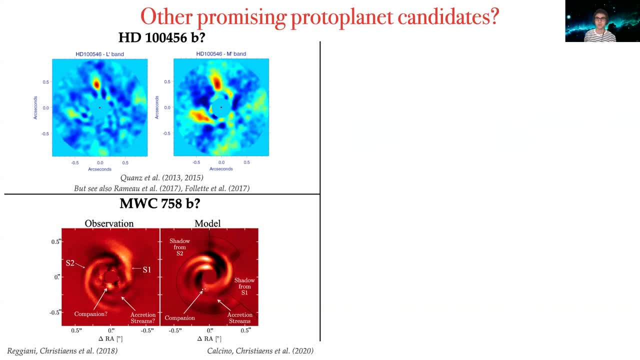 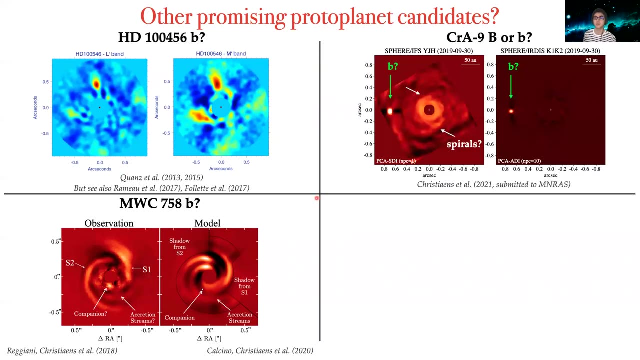 match the spirals. the planet must be located near the point source at a time step where the spirals are well reproduced. So this could suggest the point source is indeed a protoplanet. Another companion we found is in the system of CRN9.. So the companion is very faint, It's. 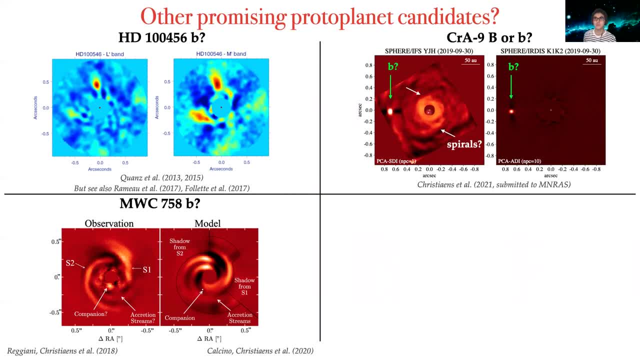 much fainter than the star, which is a NEM dwarf. It's seven magnitude fainter in the infrared, But we've found it to have a relatively blue spectrum. So it's unclear what it is. It could be either an obscured binary star, obscured possibly by an edge on disk. 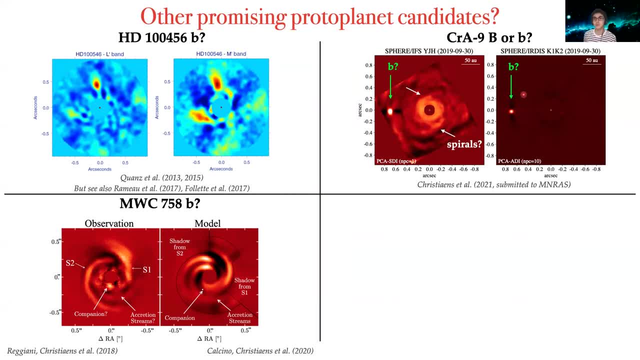 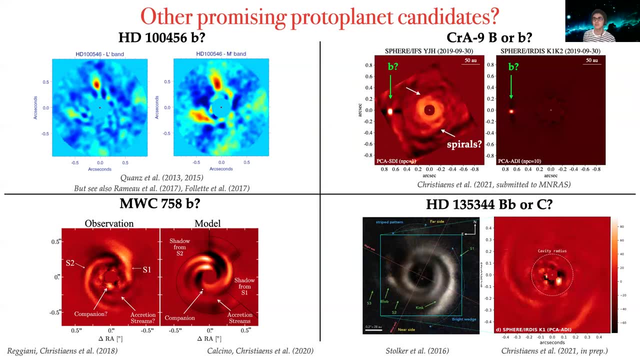 which would make it look so faint. Or it could also be an accretion protoplanet, So more observations are required to confirm the nature of this object. And finally, another promising candidate that we found is in the system of HG135344b. 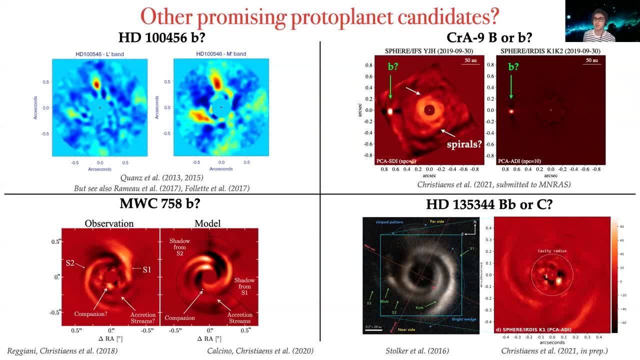 And in these polarized intensity images we see a large cavity and spiral arms And in the total intensity image we found a point source inside the cavity And again we don't know if it's a binary or a protoplanet. So we need more observations. 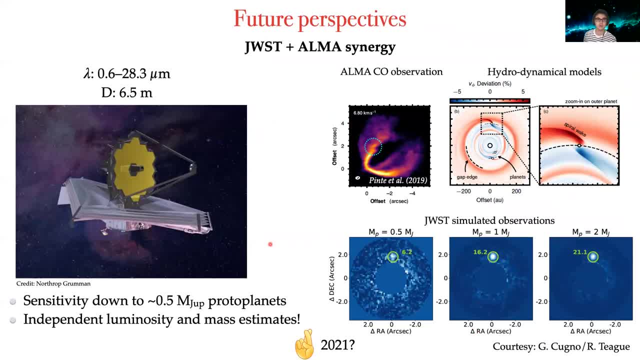 So let me finish with this, So let me finish with this, So let me finish with this, So let me finish with a few slides on the future perspectives in this field. So there'll be a strong synergy between the James Webb Space Telescope and the ALMA Subminimator Array. 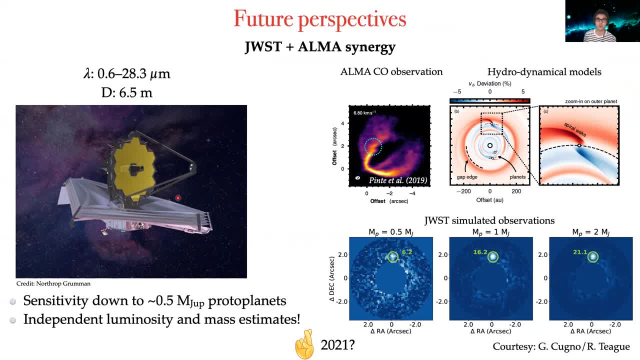 So ALMA will allow us to tell us which system to point with JWST. Since ALMA can probe the kinematics of the gas and any deviation from capillary rotation due to the gravitational pull of embedded planets, So it can help us to infer the presence of planets in 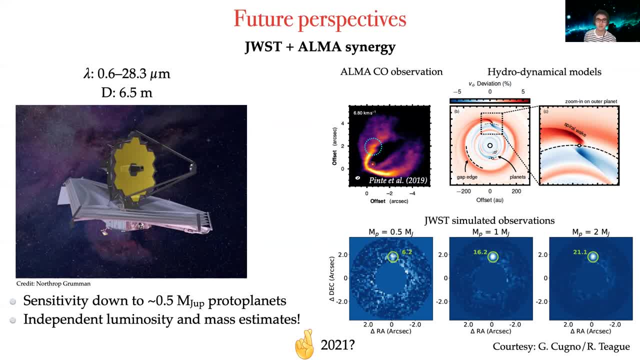 the disk. So this technique was pioneered by a colleague, Christophe Part, here at Monash to infer the presence of several limited planets and estimate the mass. And here we perform some simulated observations for JWST And we noticed that we could be sensitive down to 0.5 Jupiter. 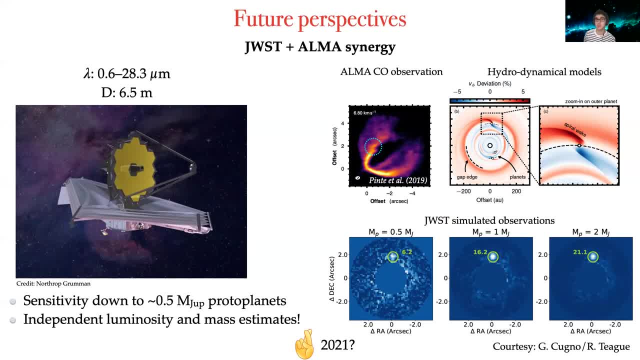 masses. So this would make the observations very complementary. So with JWST we could measure the luminosity And with ALMA we could measure the mass of the protoplanet, which would set the most stringent constraints on planet formation theories.